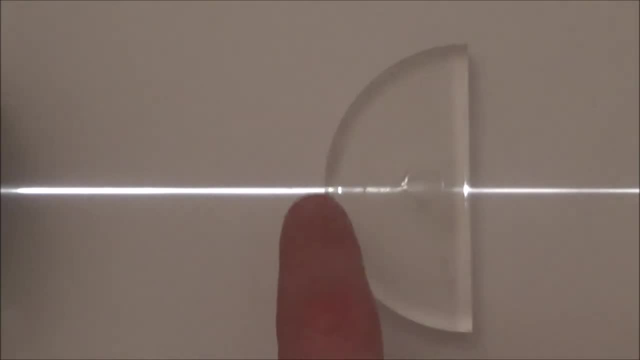 important is that, provided that we hit part of the curve in the right place, the angle of incidence is always going to be equal to zero, and what we can then do is really look at what happens to the light coming out the other side. So, as we rotate it, we should. 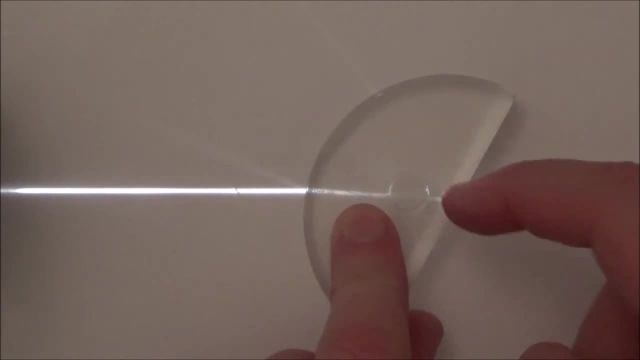 see that this ray of light moves up and up and up and at this interface here, the angle of refraction is always going to be larger than the angle of incidence. But do you think due to Snell's law, there's going to be some point where it's set at maximum and at this? 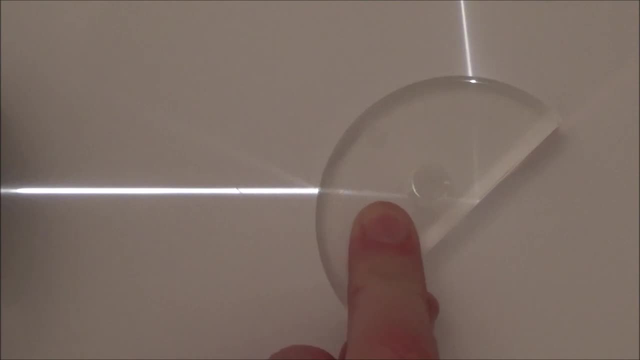 point. here, the angle of refraction is going to be 90 degrees. This is where something interesting happens. What we can see is all the light that was coming out suddenly doesn't come out of that block anymore. What's happening instead is we have reflection on the inside. 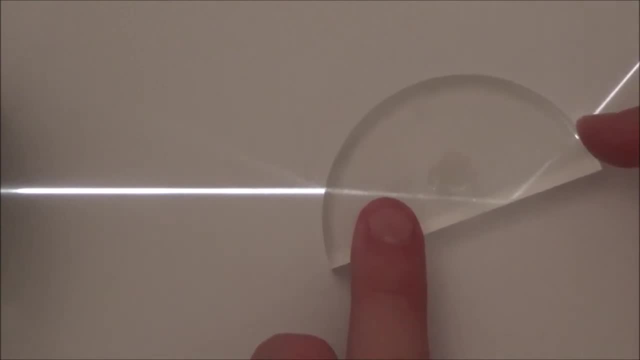 and this is what we call total internal reflection. What we can see is, as we move, that we get the light bouncing off the inside and bouncing back out again. So this effect here is really important. You might have seen it beforehand, perhaps when you're looking at a fish tank. 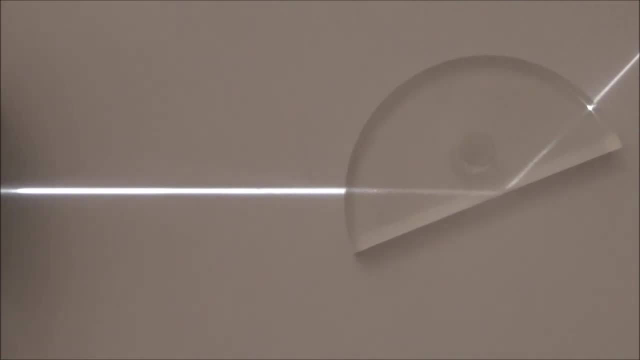 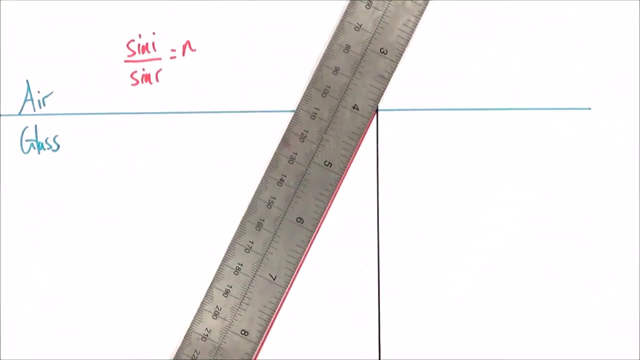 and as you look inside, you might see fish reflected on the inside. but it's also useful in optical fibres. Let's consider a ray of light that hits an interface and what it's doing is moving from something which is optically more dense, like glass, to something which is 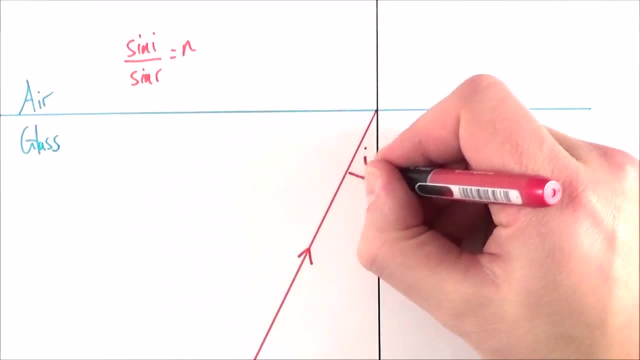 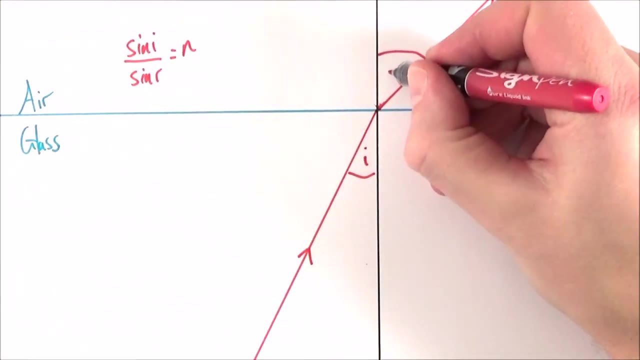 optically less dense, like air. Now here we have the angle of incidence and we also have, in this case, the angle of refraction. What we'll see is that the angle of refraction is always going to be bigger than the angle of incidence. That's all fine, but there's 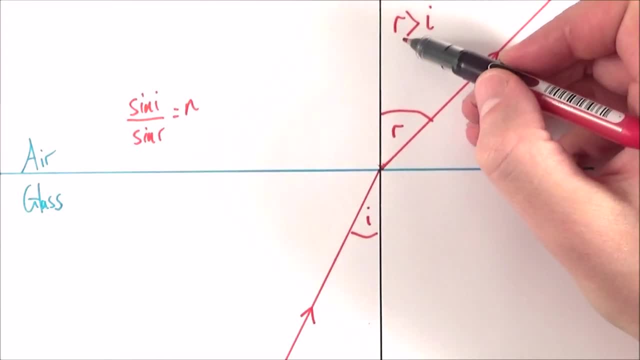 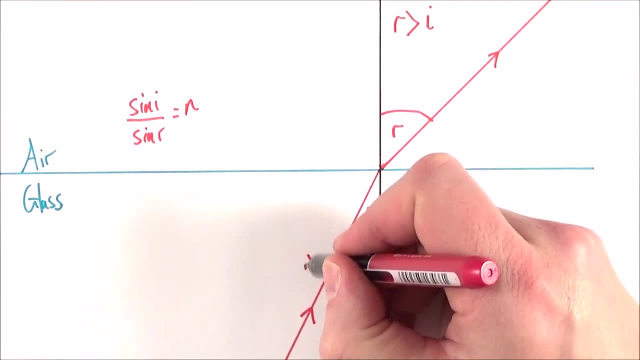 going to be a point where, if we have an angle of incidence, it's going to make the angle of refraction equal to 90 degrees. What we find, then, is that, as this angle gets bigger and bigger and bigger, there's going to be a point when this ray of light is coming out. 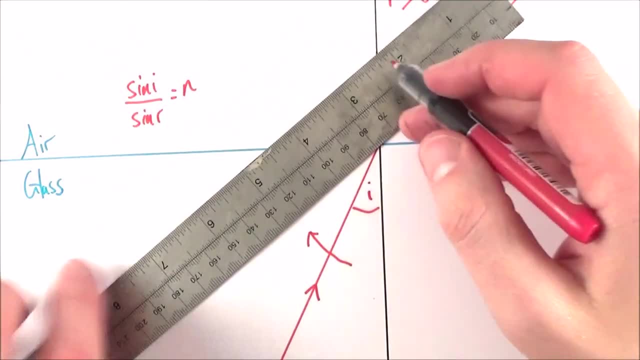 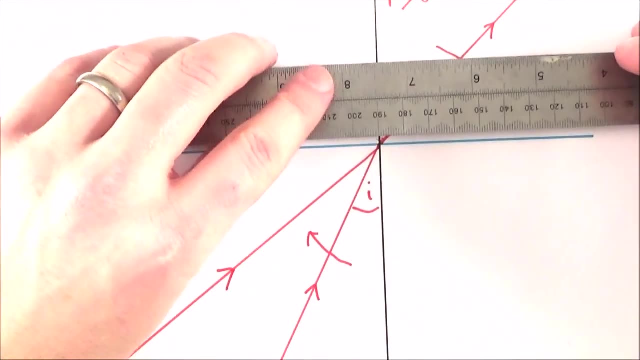 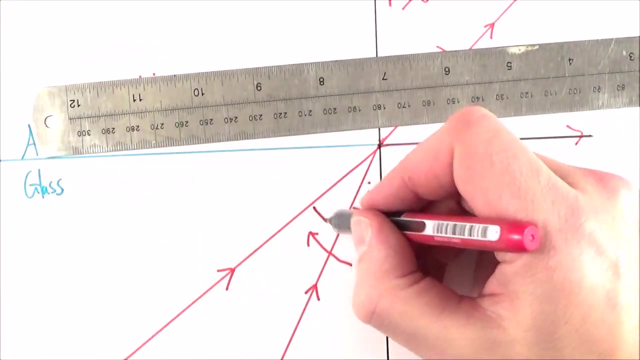 along the surface of the boundary. What we get to is a point where the angle of incidence- I causes the angle of refraction- to be 90 degrees. What we have then is something which is quite critical, and we call this angle here. I'm just going to put that in two lines. this angle here is going to be what we call. 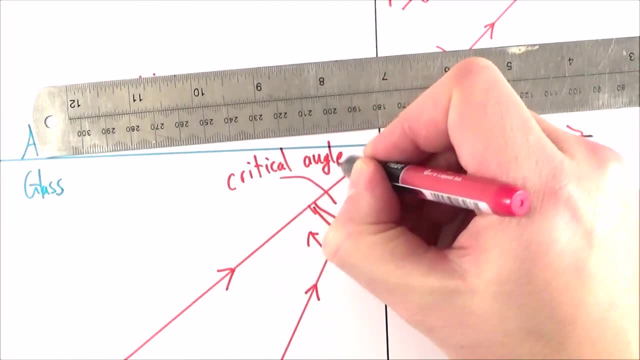 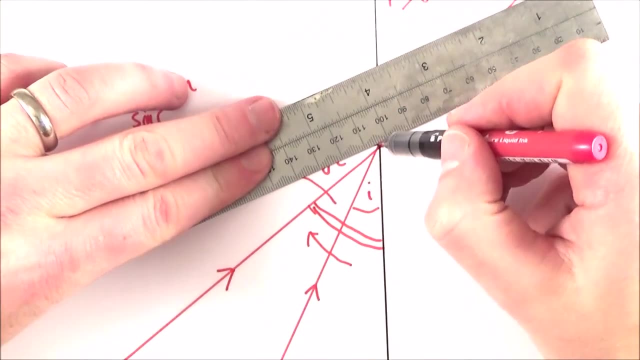 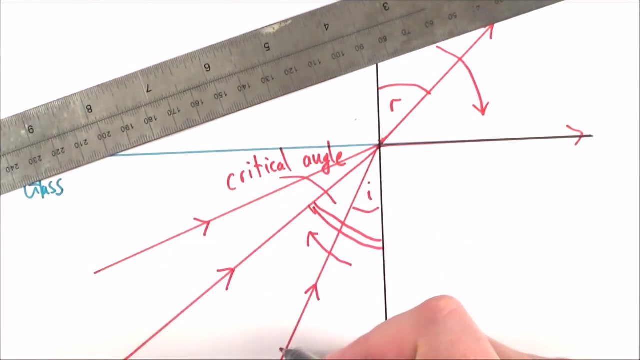 the critical angle. If we have an angle of incidence which is bigger than the critical angle, what we get then is all the lines. Let's look at the last line. That's the light that hits this point. let's call that ray one, ray two and away ray three. 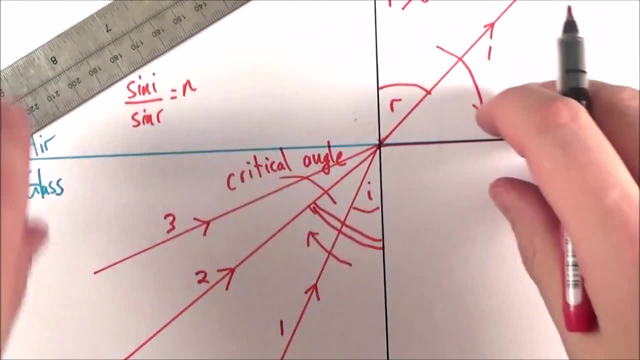 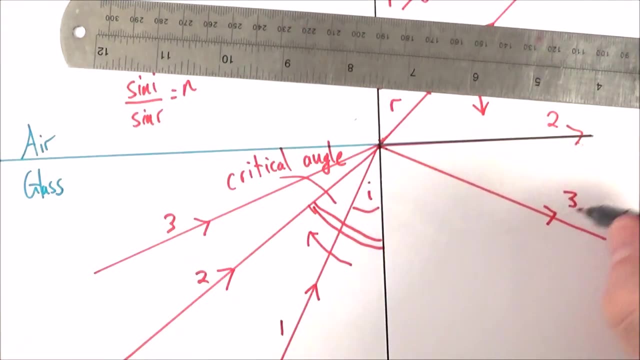 this might be ray one that comes out over here. we might have ray two that goes along the boundary At ray three. what we're going to have is all of that light is reflected inside. This is the ray three that's come out. What we have, then, is any light that hits this boundary. 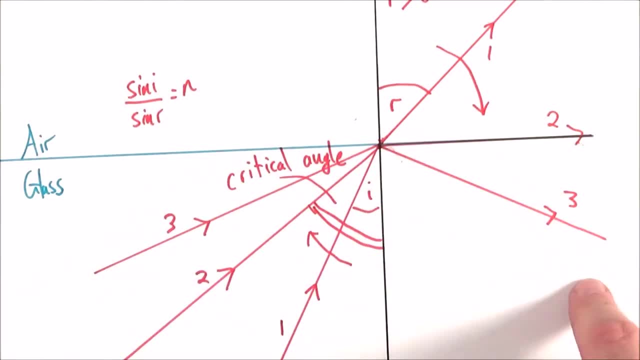 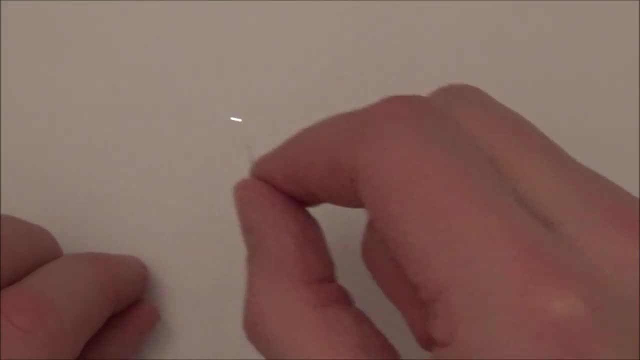 on the inside is reflected back inside behind optical fibers and how they bounce light along the inside of that. What I have here, which is quite hard to see, is an optical fiber, and if I just move it towards the lens you'll see that there's a bit of a light shining at the 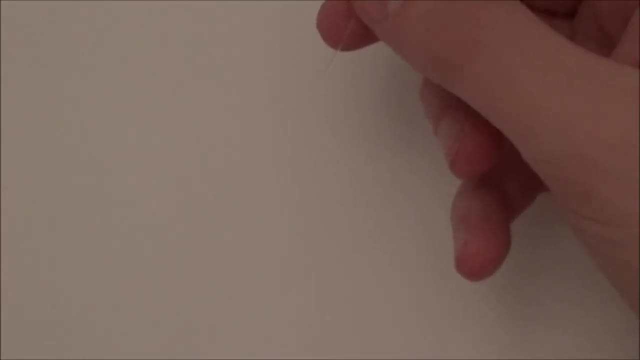 end. Now, this light source is several meters away and it's a very, very thin cable, but what this means is I can actually send light over many distances and as I maybe alter the brightness of that light or maybe turn it on and off, you can see what we can do is send signals, which is the basis. 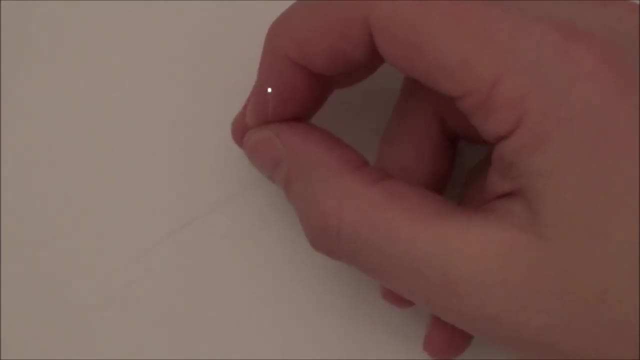 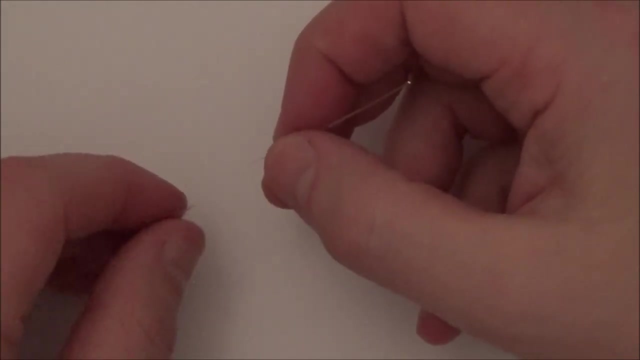 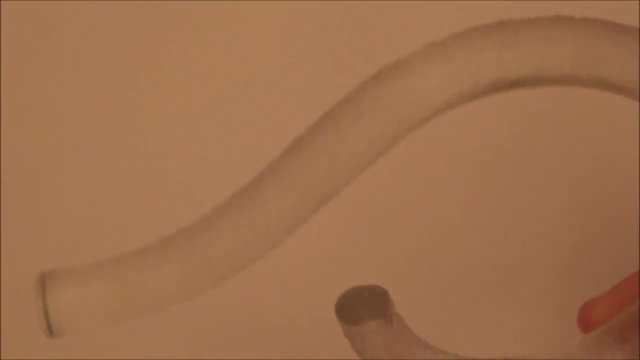 behind a lot of this kind of sort of fiber optic broadband that you might have in your house and it only works because of total internal reflection. Now, it's quite hard to actually see how that works, so I do have a larger model Here. we have a massive model of a piece of optical fiber, and if I get a torch and I 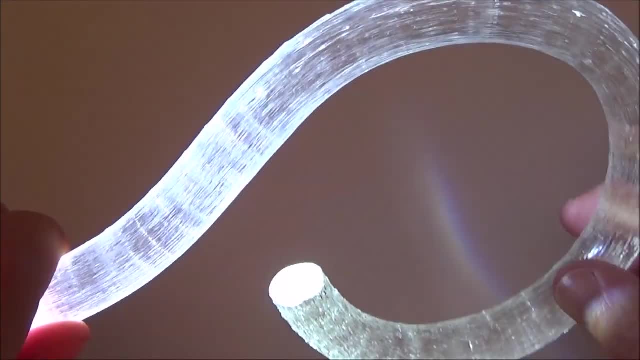 shine it down one end, we can see that there's a load of light within that and if I look around, I can see that actually a lot of light does come out of the end down here, because what we have inside is a lot of light coming out of the end down here because what we have inside is: 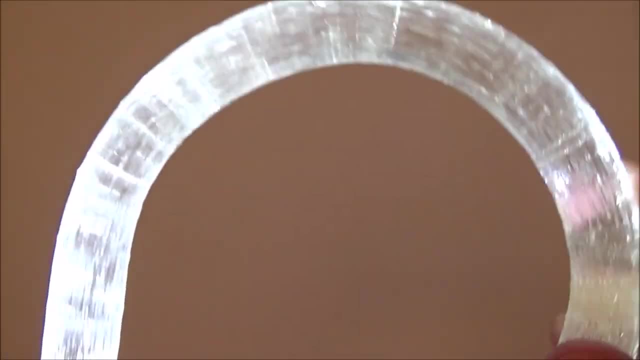 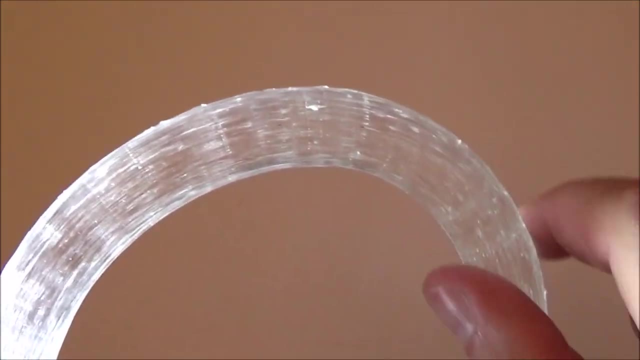 a lot of light coming out of the end down here, because what we have inside is a huge amount of total internal reflection. You might notice as well that there's- it's not perfect- there's- quite a lot of light that you can see on the outside, and this is because it's quite a steep radius of curvature here. 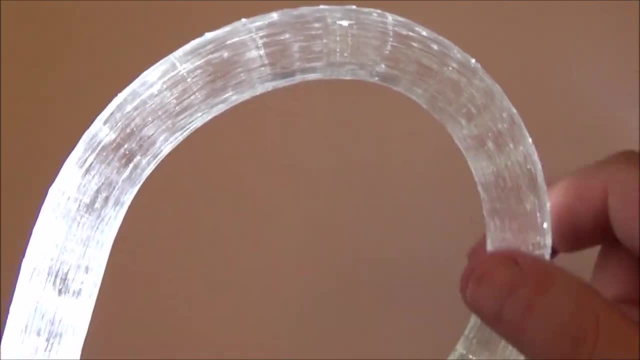 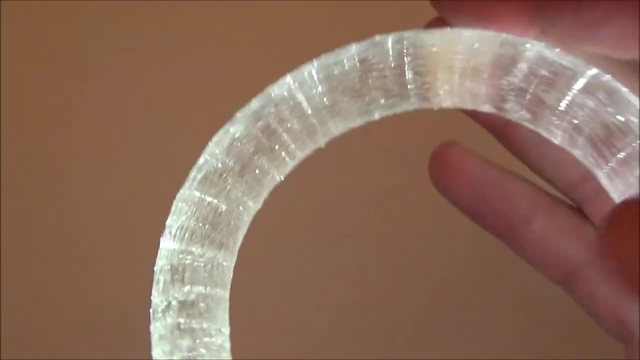 and that means that there's gonna be a fair amount of the light bleeding out and being lost from the system. Now, in reality, long optical fibers don't have to bend a huge amount, so we can have a huge amount of light that we can contain within those, and that means that we can send signals at pretty much the speed of.